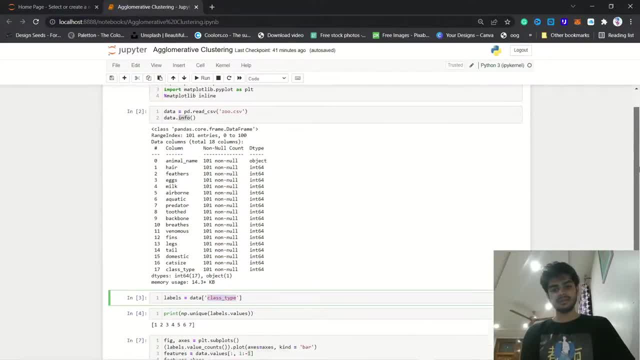 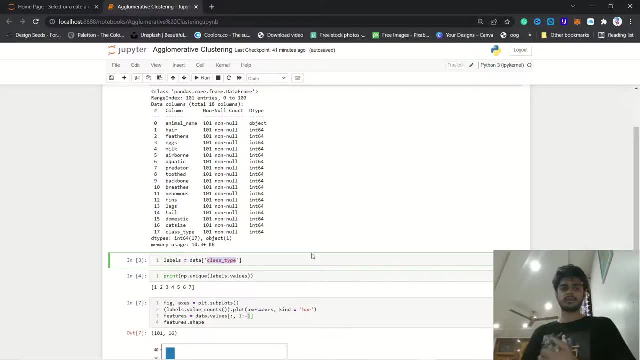 We like made labels. We like labels out of our data which is quote on quote, to work with our data, to know our data, to have something which we can use to produce in like we can use in our unsupervised learning. But again, the difference between supervised learning and unsupervised learning is that unsupervised learning doesn't have a data which is given to our with our raw data format. 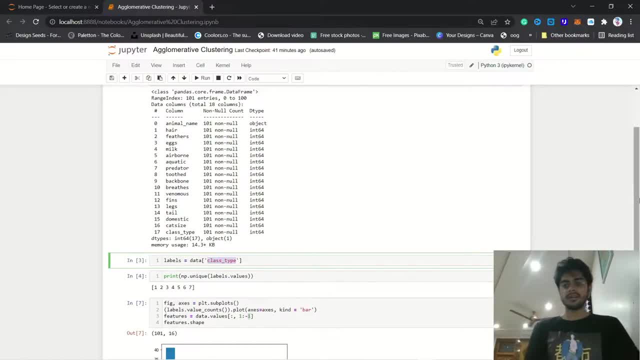 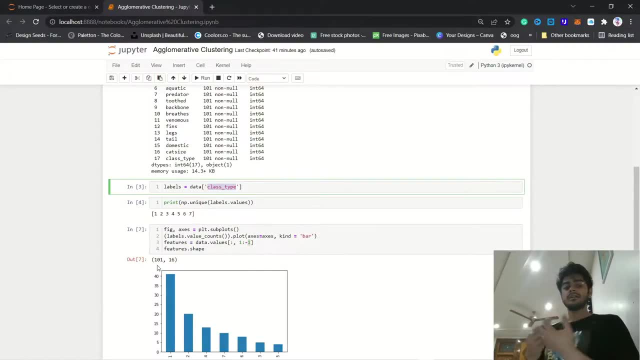 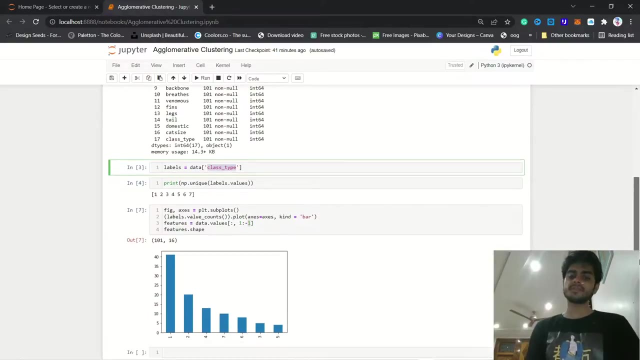 So then we printed some unique values, Then we went ahead and we worked with our data to plot some graphs and to get some features out of it and to get how many features, get to know about how many features and how many rows and columns of features we have. 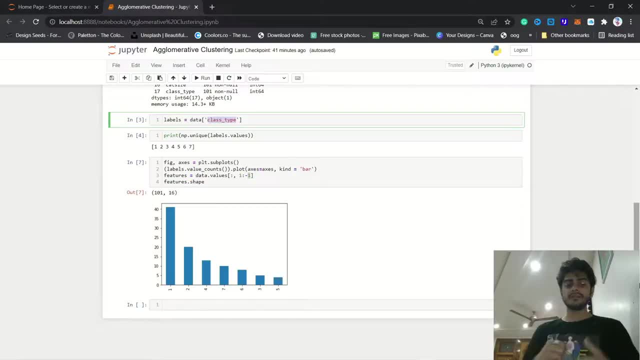 In this video. what we will do is we will go ahead and we will go and finally start coding or taking. We will take this, all information which we have collected in previous video, and we will fade it into our agglomerative clustering algorithm to 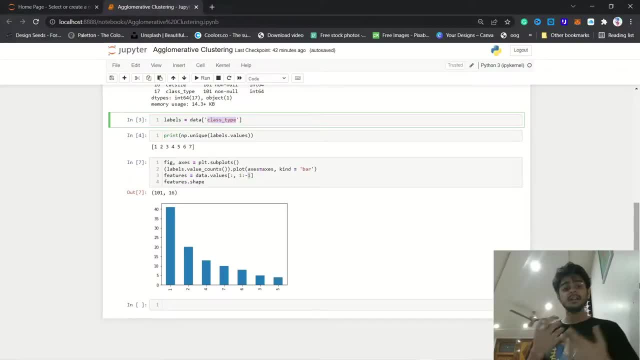 get the result which we want and to actually see unsupervised learning in action. and if you want to watch those, those videos- our first and second video- i will highly recommend it because there are a lot of information which will is useful for you and if if you don't want to watch, you can follow along. 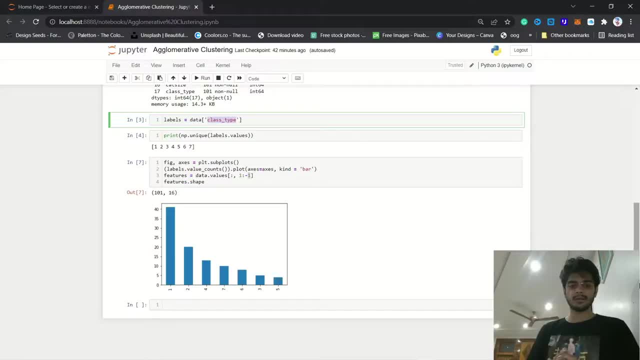 but if you want to watch it- and i will highly, highly uh suggest you to do that because that makes picture more clear- i will tag those videos in my i button and in like end card of this video. so, uh, we have done this now, as we have, as i said, that we will use sk learn library, which 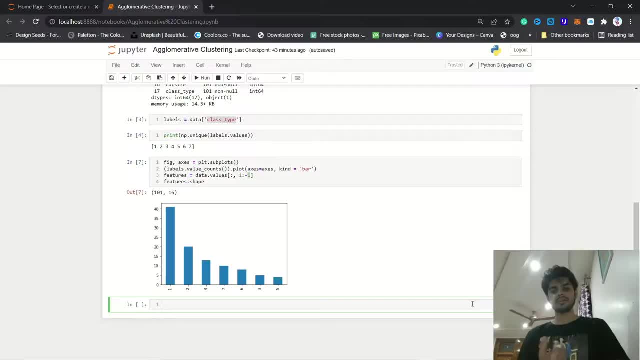 is scikit-learn library. so what is sk learn library? so sk learn library is a actually a collection of, let's say, important algorithms which we can use to perform supervised learning or unsupervised learning, and it is a very powerful library and we use like sk learn for, like clustering, like. 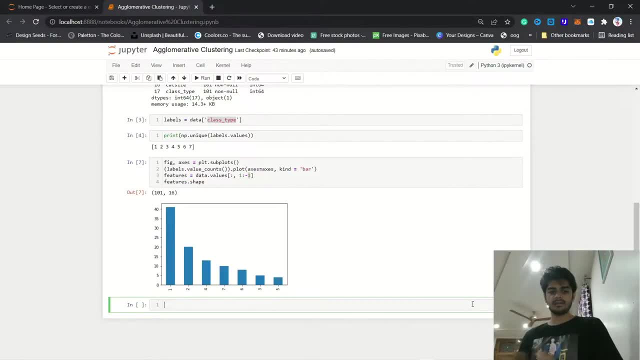 we, you can, you can do clustering uh by any number of method, but here we will use sk learn library. and again, sk learn library is very powerful library which have a collection of algorithms which can, which we can use to perform our machine learning tasks. so, uh, we will say from sk learn this: 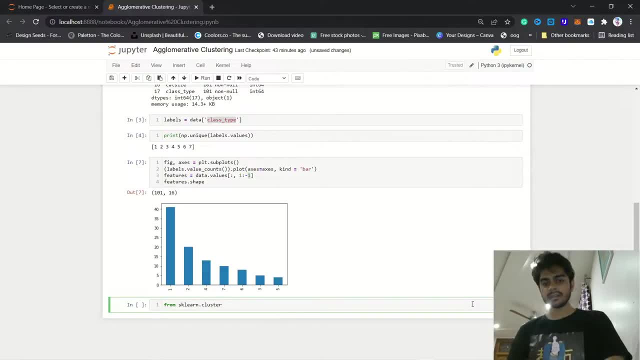 dot clusters, because we are working with clusters, we have a sk learn library which have a cluster, which have the property of agglomerative cluster. we will say: from sk learn, dot cluster, import agglomerative. and we can say one more thing: from sk learn we want to have like, if we like, uh, use clustering as we have discussed. 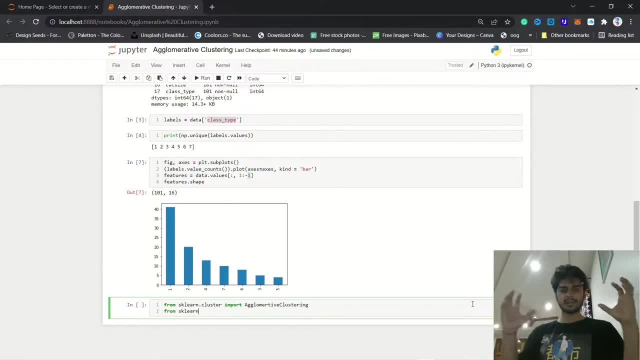 that we divide the like uh whole cluster into small parts, or we uh take small parts or sum them into a bigger part. so if you can like, put this information into perspective, you can see that there must be some difference, like there, there must be some distance between two clusters. let's say: 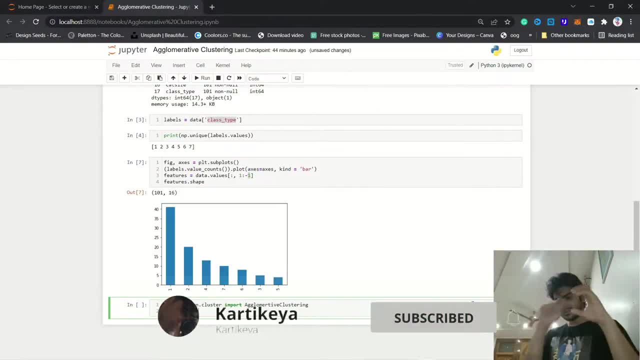 there is one cluster, there is this cluster, this thing, this here is the distance between two clusters. let's say this is one cluster, this is one cluster, this is one cluster. so so the space between them is the distance between those clusters and if we are saying that we are merging, that we have to calculate the distance. 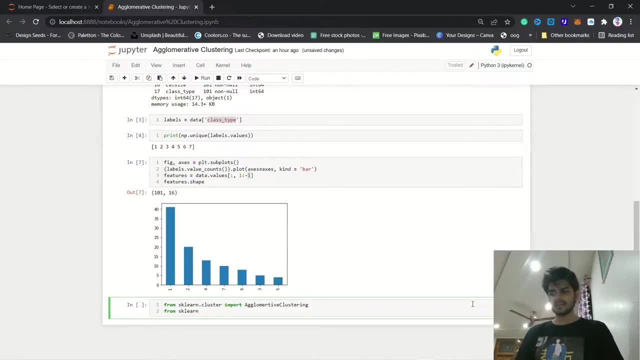 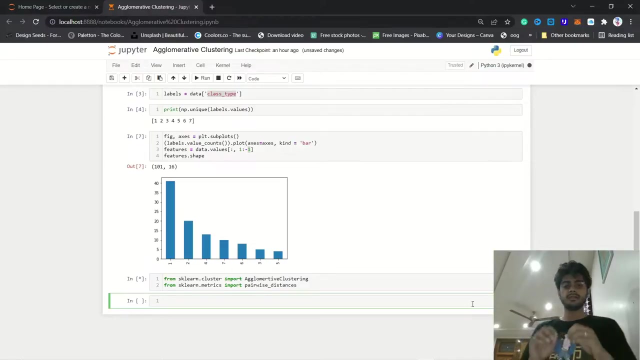 so we will import a pair visor in this distance property from from sklearn which comes from sklearn dot matrix. import pairwise distance, pairwise distance. lets import it first. it can take time and if you have not like, if you didn't have your sklearn or sklearn library installed in your jupyter notebook, this can show error, because 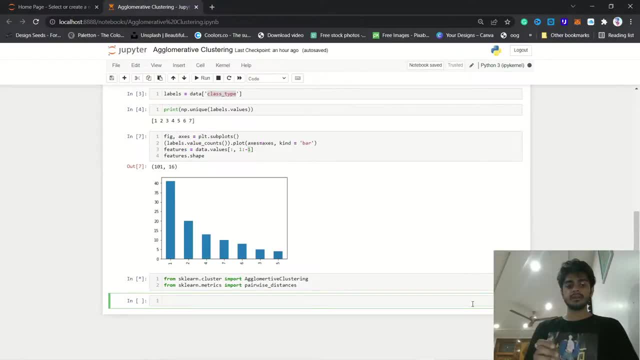 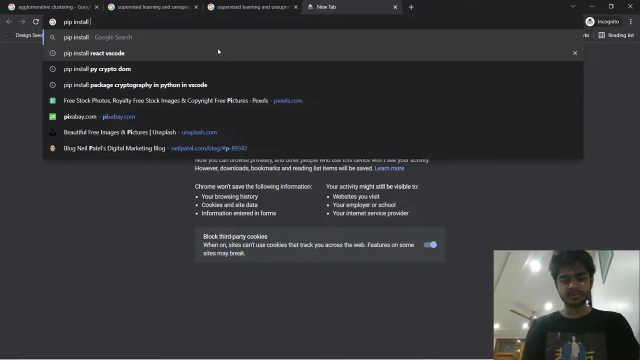 you have to first install, or pip install, your sklearn library. so let me show you how to do that very quick. so i have installed that. go ahead and, like you can say, pip install sklearn and it will give you the installing sklearn library and how you can install it. 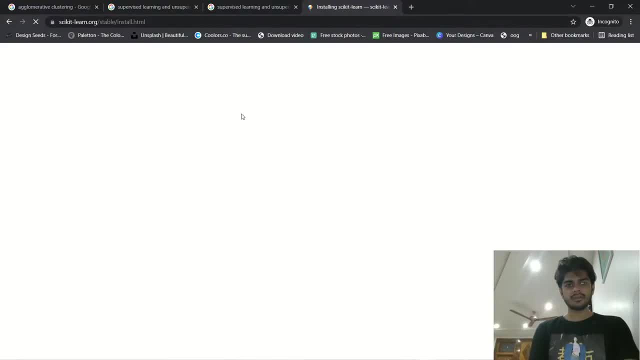 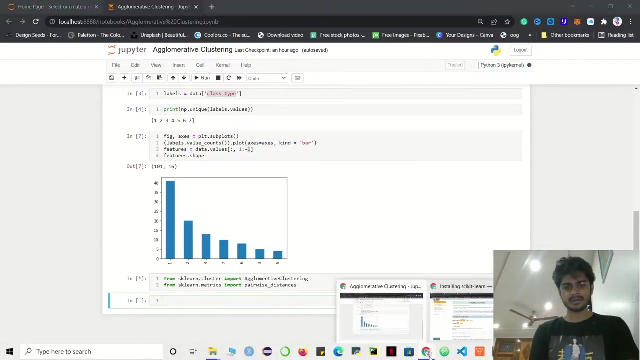 and how you can install sklearn library. so or you can follow this documentation from here, or you can go ahead and write: pip: install your library in jupyter. its taking time, lets see. so it is importing right now like our. okay, there is some error here. what is that? 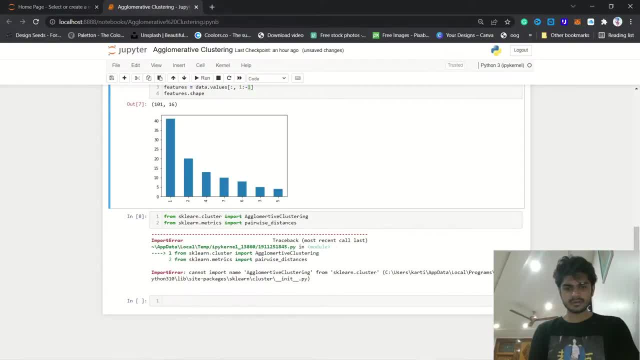 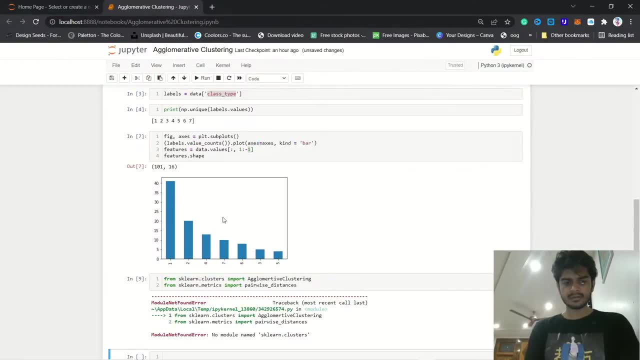 error dot. i think that is clusters or what. let me check with clusters. okay, let me check again with spelling mistakes: a-g-g-l-o-m-a-r-a-t-i-v-a. so like, be careful with your spellings because, yes, this can give you error again. this should. 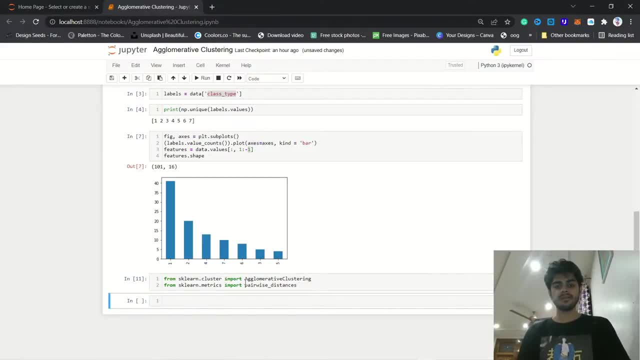 be clusters. so yeah, now we have successfully imported our two like features from our sklearn library, now work on it. let's work on it. let's say we have a model variable and we will say that that model variable will take, will take agglomerator. may i have to be extra clear? careful with the spelling. 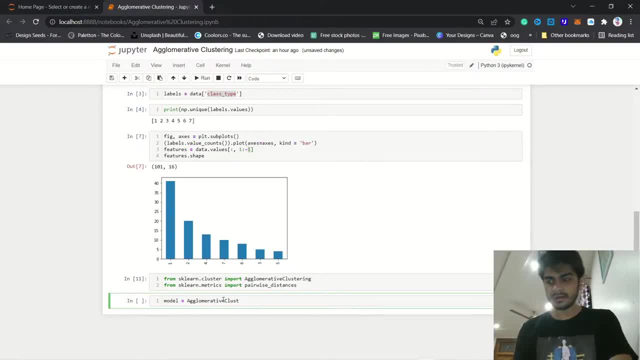 because that can show error. it will take agglomerator plus string and it will take n clusters. n clusters is how many clusters you want to take. so let's say we have a model variable and we will say that that model variable will take seven clusters, and then we know that every it will take lots and lots of clusters. 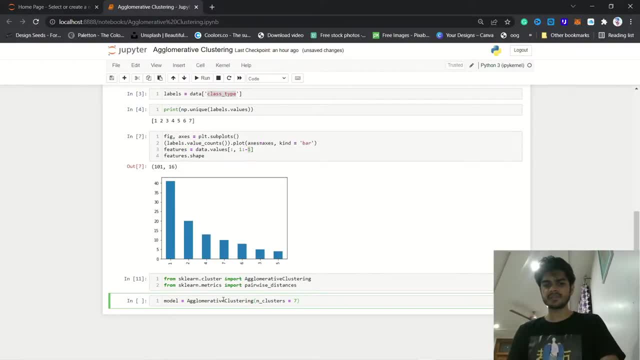 we know this one of them is going to change whatever element. so, ah, let's see. so, uh, one, that whole set of your水 and it is. you can add your entire, like landscape. so let's say, let's say I have two sets of cluster. so I'm going to say here, i think it will take. you a set of cluster. we are going to say I have built this evidence here for some data, like your data set to divide, and I will go for seven clusters so you can play with. this says actually parameters which you can play and see how, how good your data sets turnout. 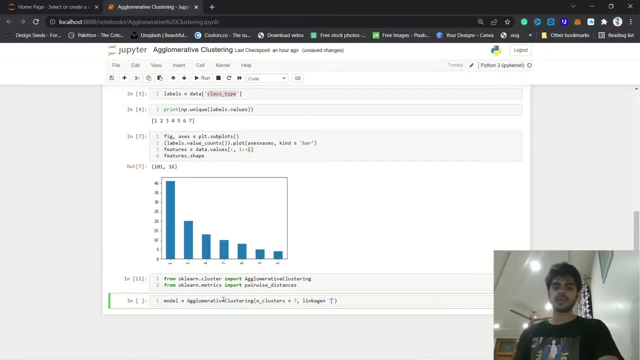 these parameters in very diff when you search for agglomerative clustering. but yeah, in very basic information this is like number of clusters. you want linkage. what type of linkage you want? I'm going for average, like I want average between. I want our linkage to be of type average. then I will go for. 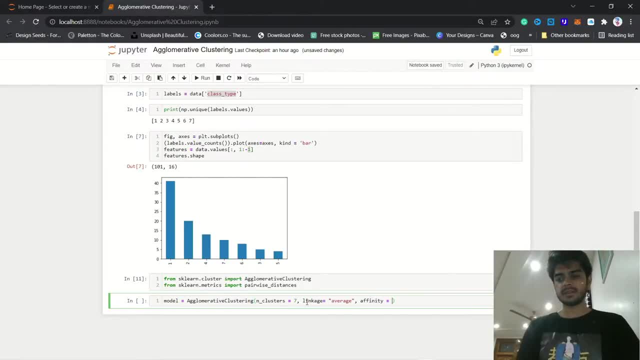 affinity, like. affinity is basically with like. we have a sign property, we have cosine property, trigonometry, because, again in in very broad perspective, all we are doing is performing some maths with our data set. like to be very honest, machine learning is just a combination of matrix statistics and probability to 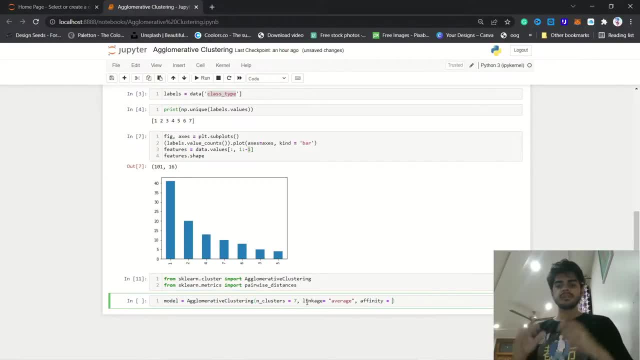 get predictions from our data set. so we are just performing mathematical operations on our data set and cosine. if you have basic understanding of trigonometry, you know what cosine is, sine cosine and tan values. so we are saying that we will go for cosine affinity again if you want. 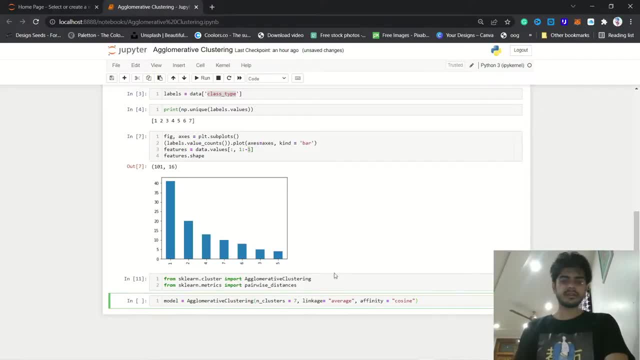 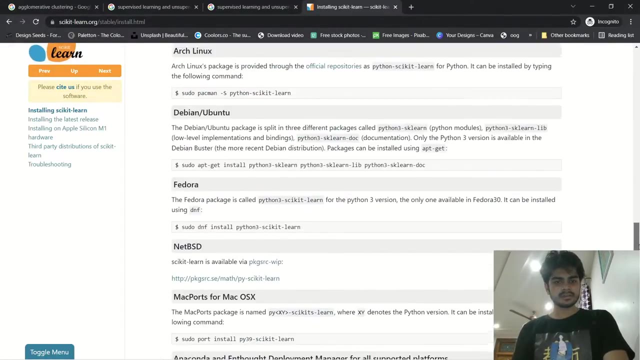 to read about this in depth. you can find that documentation on like sklearn agglomerative cluster. but again, if you want me to show you here only let's go for that. so here is how to install your sklearn cluster. this is a documentation log or documentation to install, and here is how. 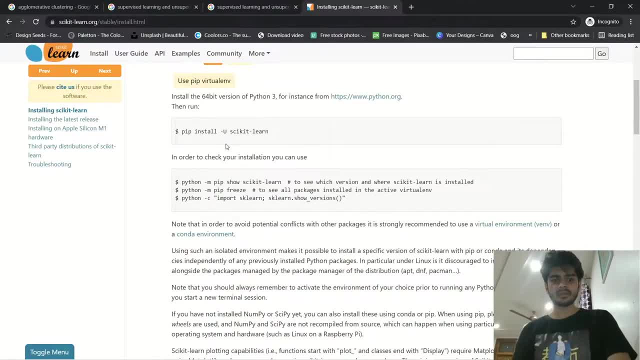 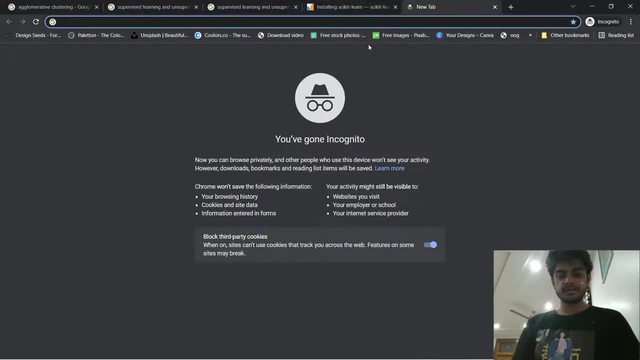 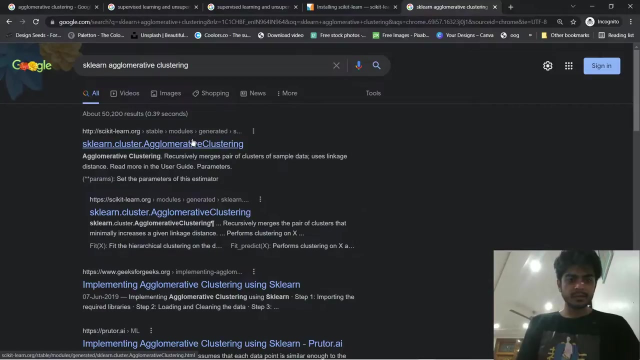 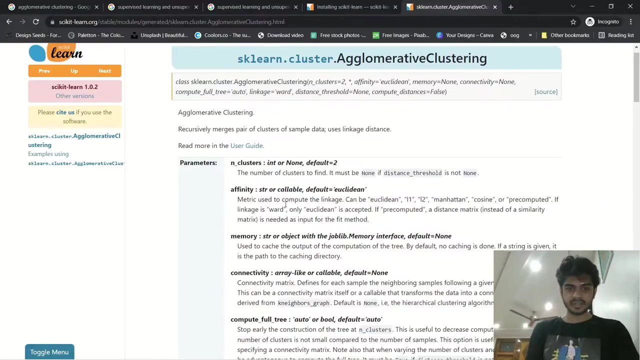 you can pip install. you can pip install by saying: pip install u sklearn. you just should install your sklearn array and let's say we want a documentation on sklearn, again with a spelling merkti. so yeah, by default you can see that nclusters is 2, Affinity is a string or column will. 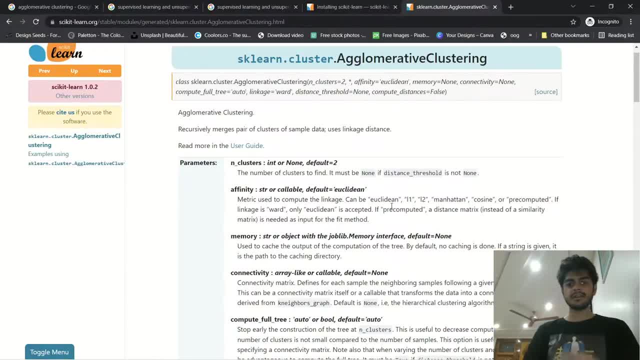 matrix. matrix is used to compute the linkage that can be Euclidean. Euclidean is different, like between: if you have like radar distance formula, you know what is a euclidean with an euclidean is a string and if you have a red distance formula, that's be formula. it is in the root something x minus some value of square and plus something, something. 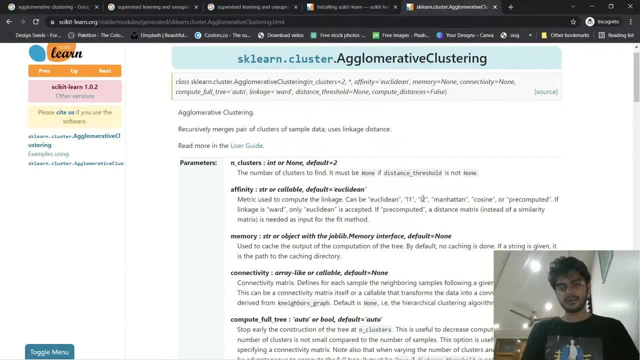 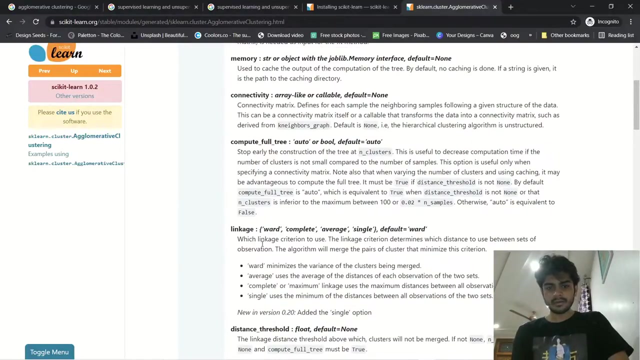 something. then these are value l1, value l2, value, Manhattan value and cosine and three computed so you can use between like from this and it actually calculates the linkage between your data. then here is what I have used linkage like based on your criteria, like you can use the linkage I have. 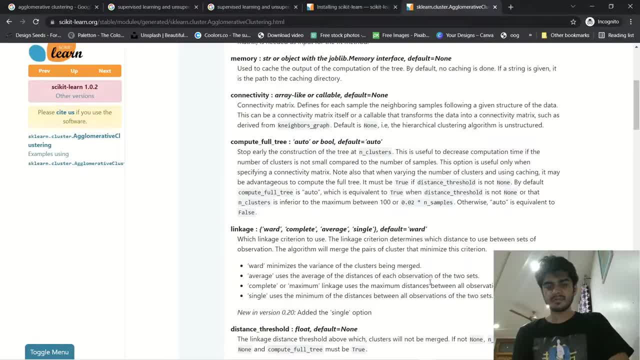 used. average uses the average distance of each observation tip in two sets. so I'm like the average between two data sets. so there is that. so yeah, if you want to read more about it, here is the documentation, which is psychic dot as I get learned or towards here, or you can google it like how I 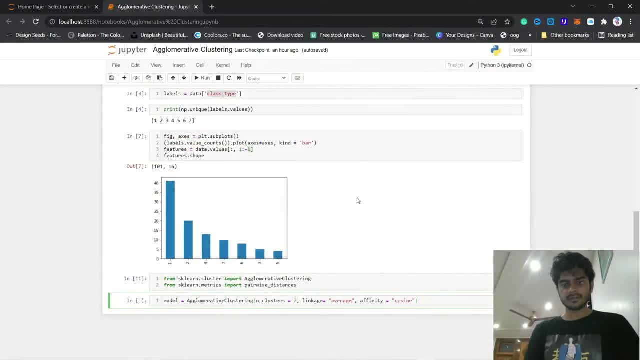 googled it and you will get to this documentation. so I think now you understand what is linkage in infinity means. so I'm making a model which will take a parameters of n clusters, which are seven, linkage like average and affinity of cosine. and now let's go and fit our model and we will say: model dot, fit features. 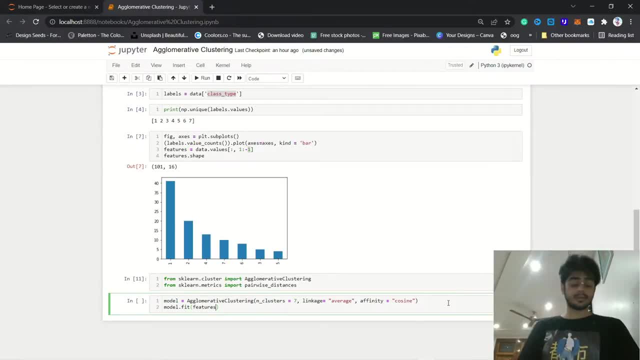 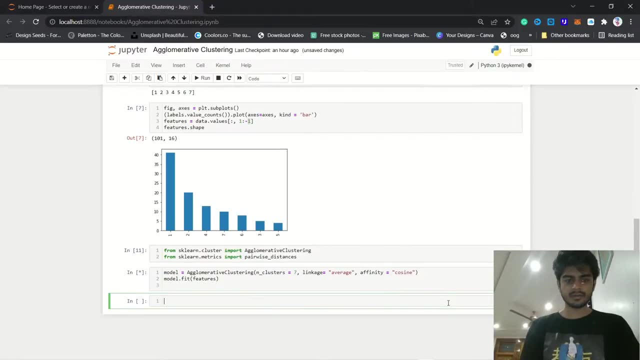 and let's first favorite our model. so this will actually take features and try to fit our model with these property which we have to get it and then after that we will go for label, which is here. after putting that data, we will take label and we won't save it. 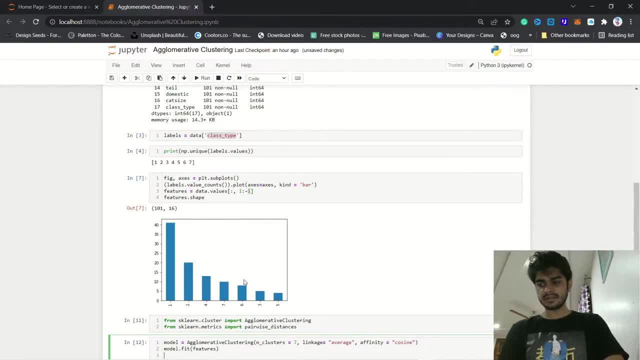 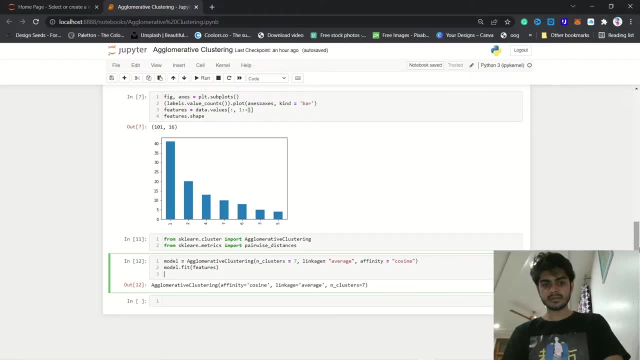 someerme, sometimes when, when some will see how we can perform some operation so that we can get some useful information out of this code which we are writing so like. I think our modelfit worked and let's go and take label, modellabels, modellabels, and we will say that. first, showing the unique values. 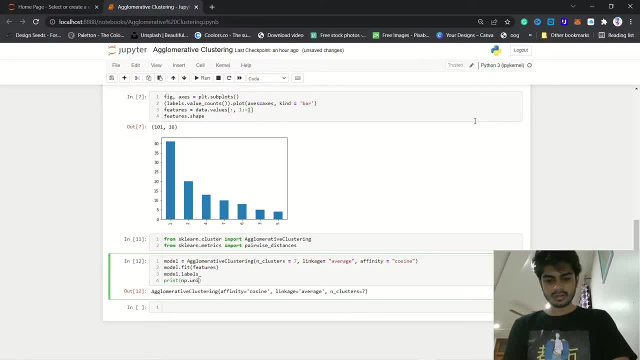 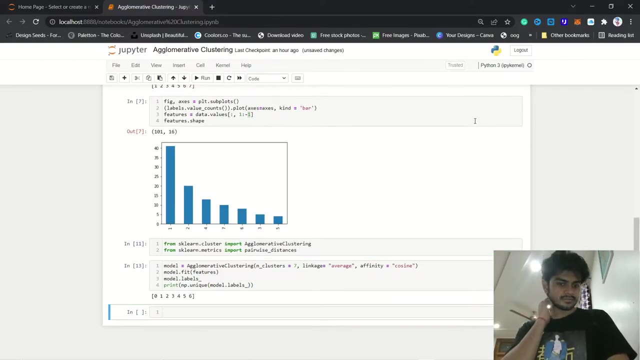 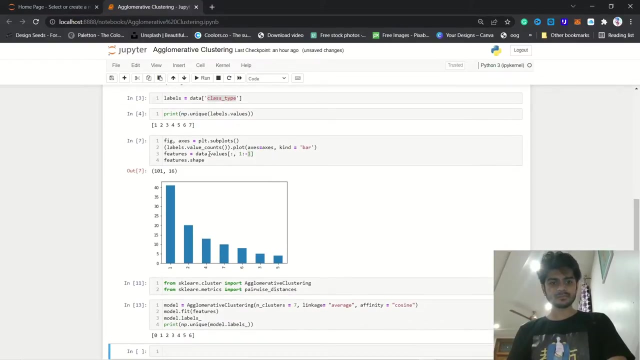 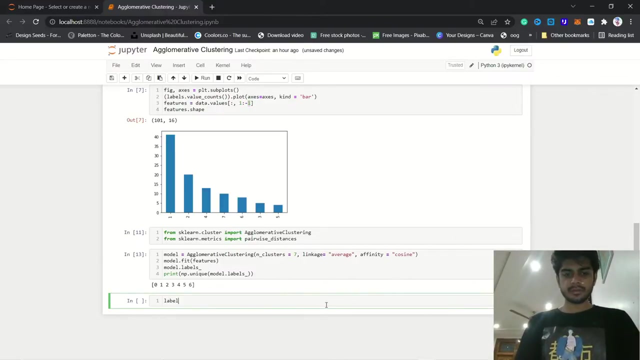 lpunique and hue unique and modellabels. so again we are getting the same information, like 1234 as previous, and these are the unique values we cross checked. let's say we want our labels to be labellabels and like: see, I am performing all these operation to actually get the unique information out of our dataset. 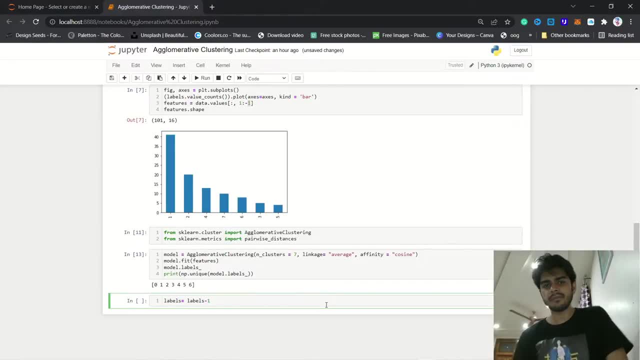 and this is like when you get different kind of dataset, you have to perform different kind of feature engineering, exploratory data analysis, EDA, which is a fancy term to say that find some useful information from broad perspective of data and just find some data which we can. 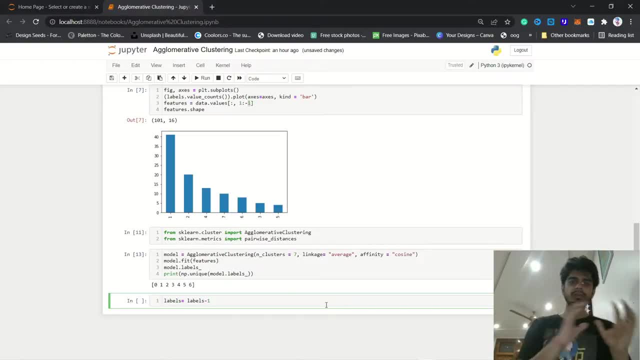 use to make our machine learning model to all EDA, which is exploratory data, analysis and feature engineering. all these stuff basically means that filter your data in such a way that you can make a use out of your data and filter your data in such a way that you can. 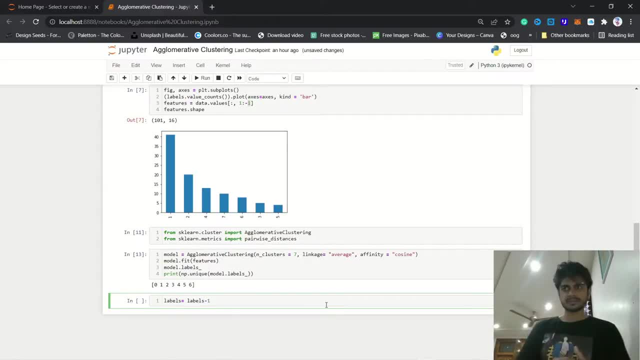 useful machine learning algorithm out of it. like let's say, I have a roll number, I have a name of a student, I have a age and sex and everything like let's say in which school he goes and is there, like he is a single child or he has a sibling. 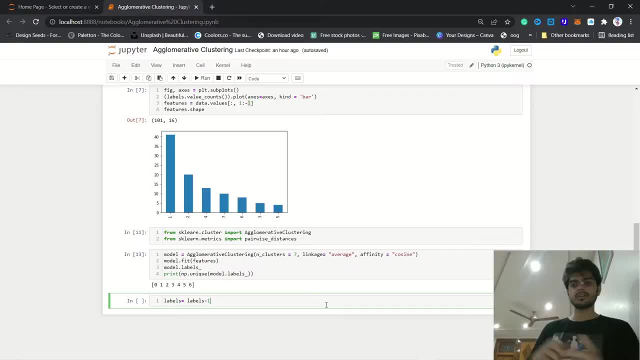 or he's a single mother, like he has a single mother, or a single father, or like both parents are there. so, if we have a these kind of data sets, like we have all the information of this and we want to, like give some, let's say, benefits, let's 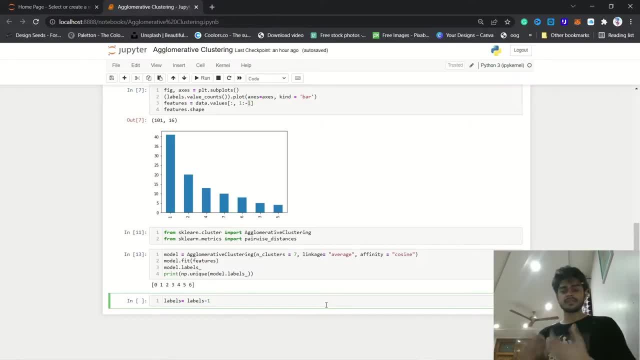 say, we are distributing some benefits which we came, which we receive from our government, to distribute between students, how we can do that in that case. we don't want any information that, whether like he has a single mother, single father or anything like, we can use in some another form to find some another thing. 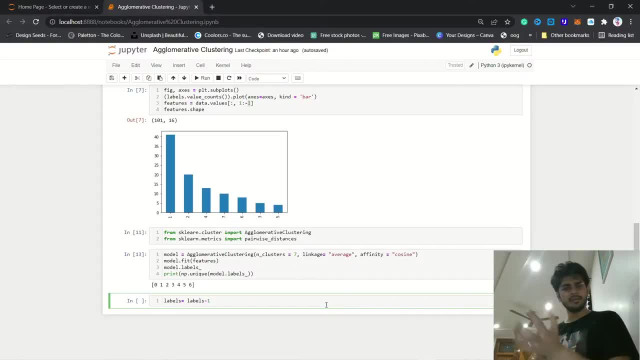 but in this case, all we want is row number and we want a name for our student to check whether the like a beneficiary got the benefit of that uh, like a scheme which government ensure us to provide them. so or, in summary, all i'm saying is find. 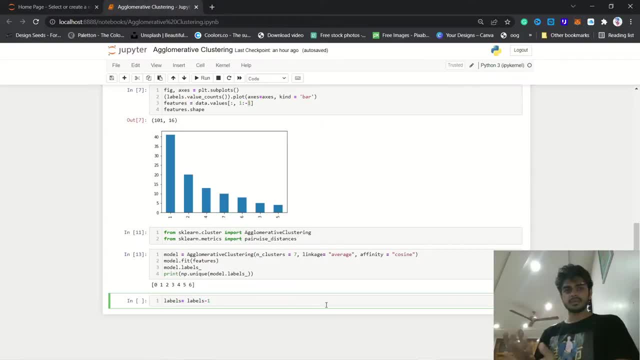 some useful information which we can use to make a good and a meaningful machine learning algorithm and we can find some data out of it. so all ed and feature and engineering in explorer, like in machine learning, boils down to this. so, uh, yeah, i'm saying that, uh, we want labels and 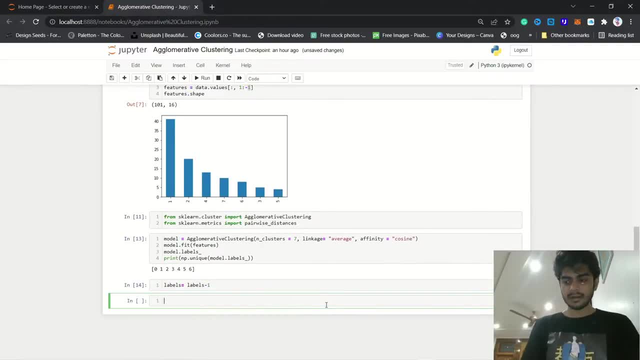 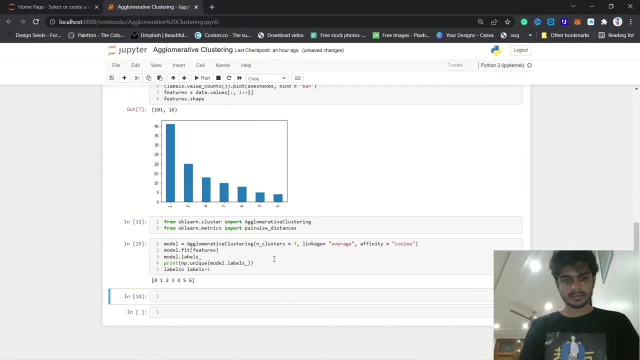 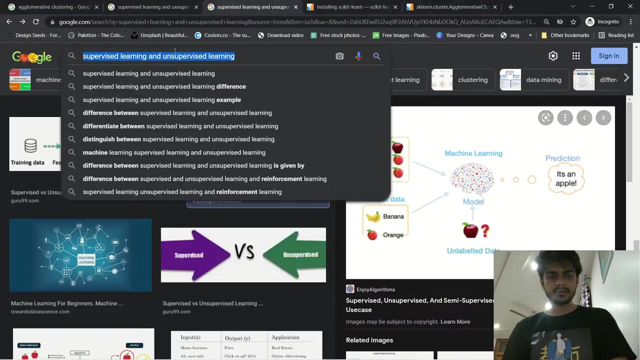 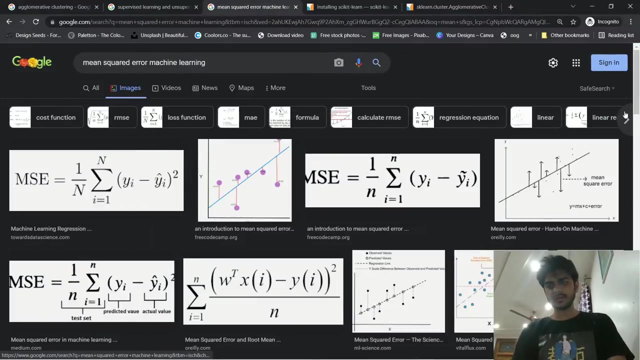 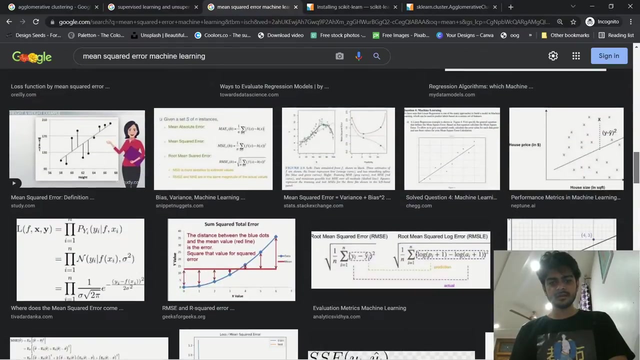 labels will be labels minus one. um, okay, now we want a mean square. what is a mean square? uh, error. what is a mean square error? let me go to our this and let's go: square machine. okay. okay, this is some fancy diagrams. okay, these are the formula of mean square. 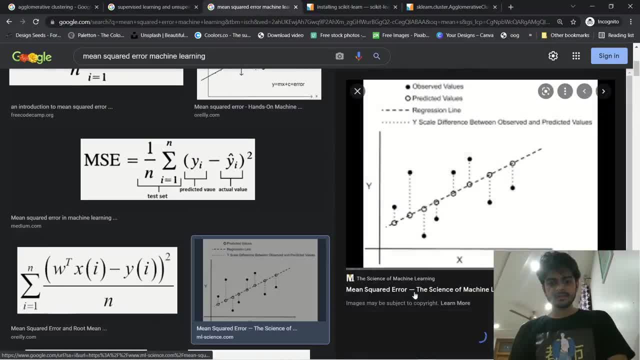 error, but, in very basic sense, let me tell you what is this. so, as you can see that these are our values present. okay, these are predictive value, which we thought that they will get. okay, this is in the context of supervised learning. so they are showing regression line. these are regression line. 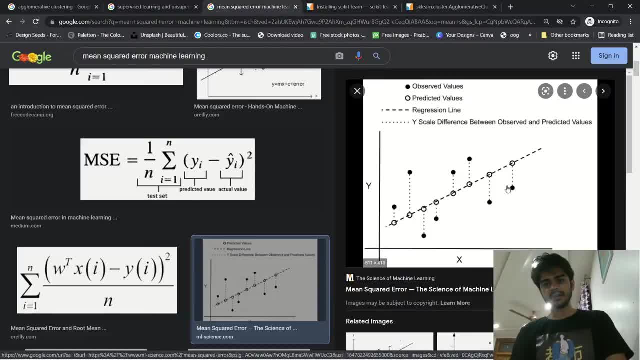 like these are the difference between what is a predicted value, what is a real value. so all you can see is that the difference between these like predicted and observed value, there is a like, some distance and some sort of error which we are getting, and that is actually. 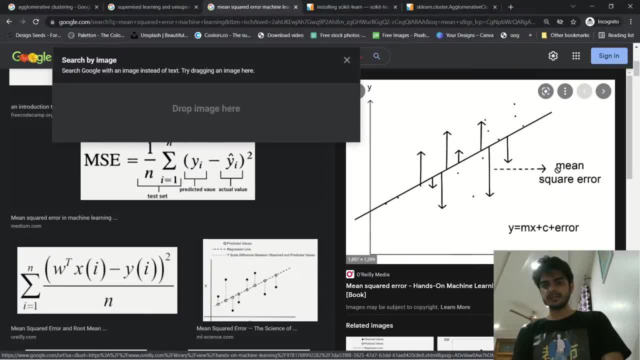 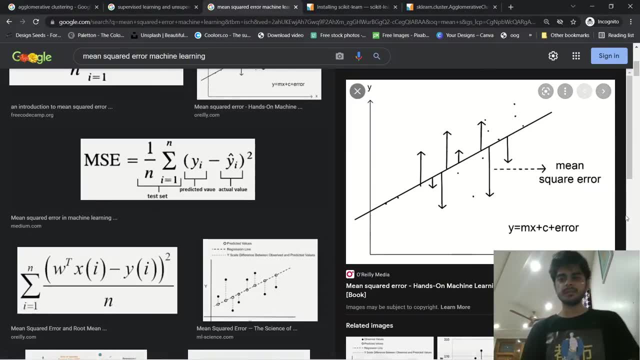 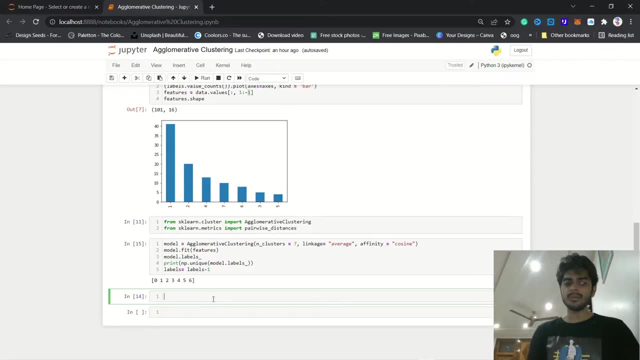 known as mean square error. like we want our error to be minimized, so we take the square of our error and then we take a mean of that value, so that we- that is known as mean square error, and we do that to minimize the risk of our data and the error present in our data. 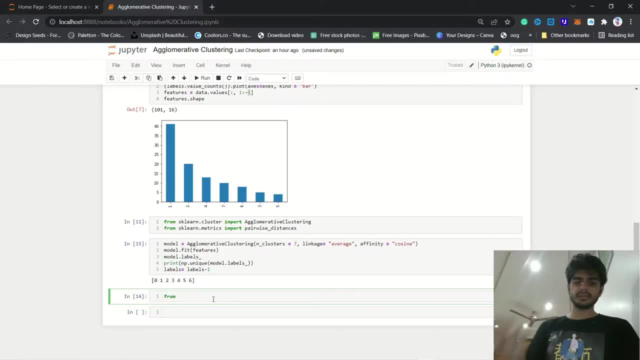 so we can get some good machine learning and significant model out of it. so we will go again from sk learn, dot matrix again. the matrix uh is a library from sk learn which is in very basic sense uh we use to perform mathematical, complex mathematical and uh operations. 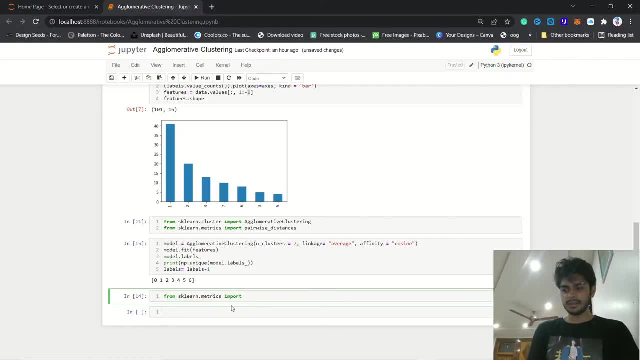 so from sk learn dot matrix import. we want a mean underscore square. let's give you a reading again. be careful with your spellings or if i show errors. so we want the prediction for our like how good our data or machine learning algorithm is or how good our 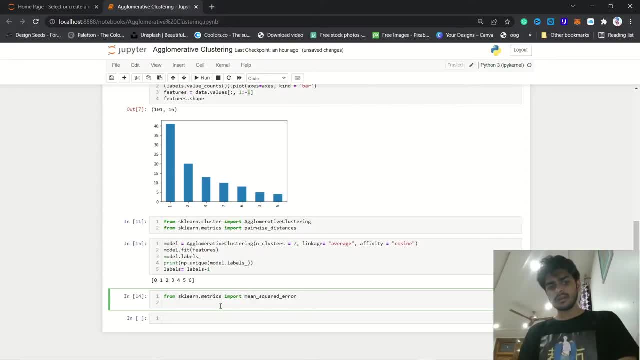 algorithmic clustering is. so we will uh say: okay, i'm taking this mean square error, give me a score out of it of all this data. imply this to all this data and i want a score, so i will. we will go and say in the mega score variable mean, let me first import it. 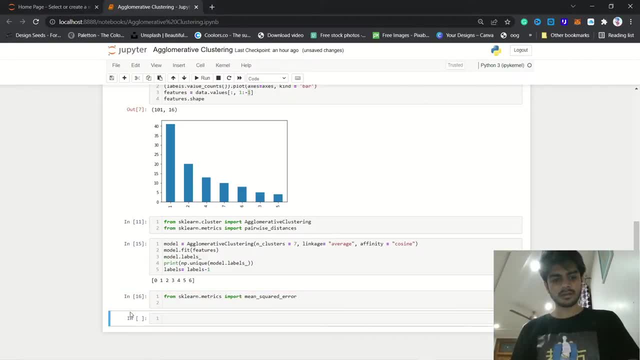 if there isn't any error, then we will get here only okay, we successfully import it it. so i will say score is equal to means, means. again, we will take labels, which is here okay, and we like, if you want to see where the labels came from, it is. 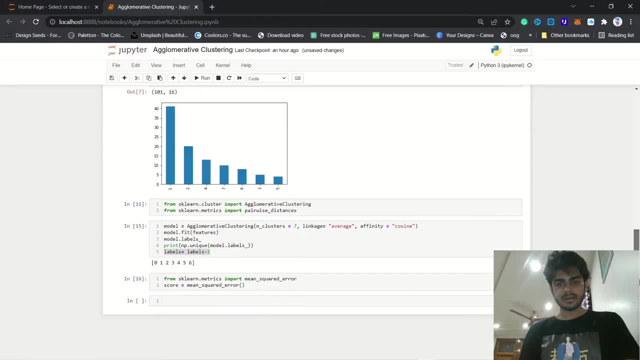 here. okay, we will take labels because, again, as you can see here we are working here with features and labels, so we will take labels and we will take model model. so we actually took our, like, we took our uh data, we feed it into our model uh variable and we put that up with that. 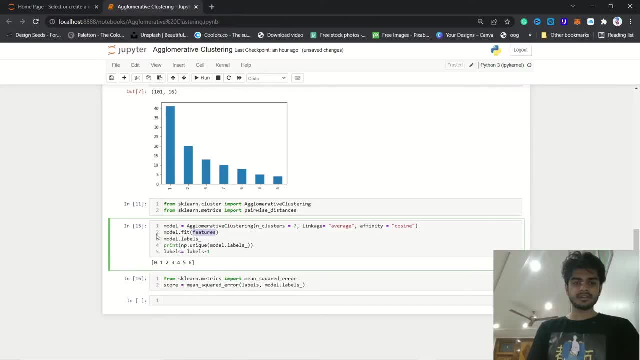 data to our we fit uh features to our model fit variable and we actually took label and we have given that value to our model. then we said: uh, okay, uh, we have this modellabels uh, which have unique value of this and their labels is equals to labels minus one, and again, we are taking that only. 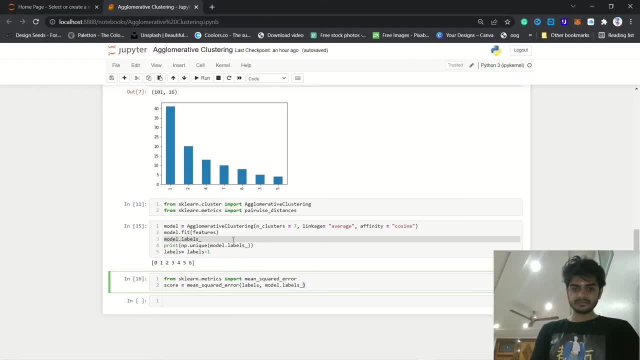 we are taking labels and model dot labels, uh, which we have, and then only that is За, will compare the score between here and we will say absolute, absolute error. what is absolute error like it is like these all terms from, comes from mathematics, uh, so i'm 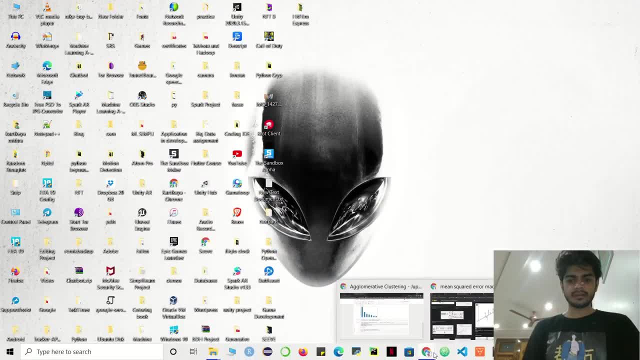 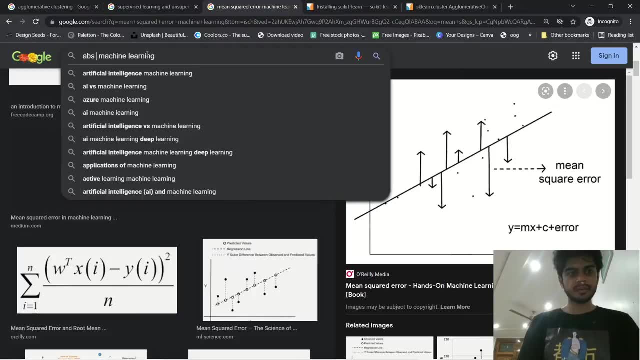 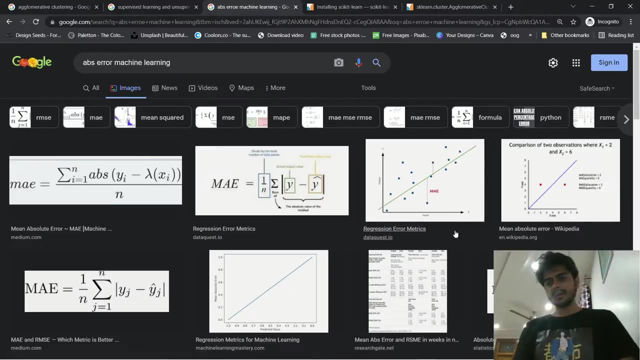 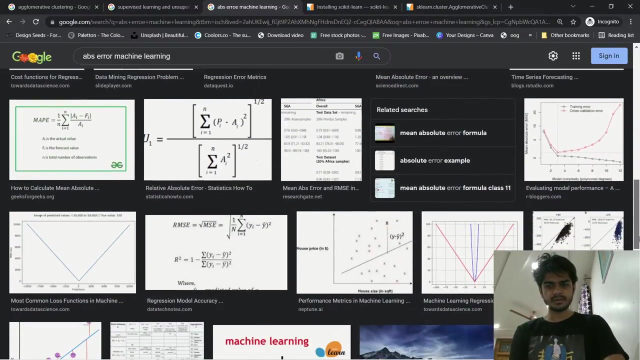 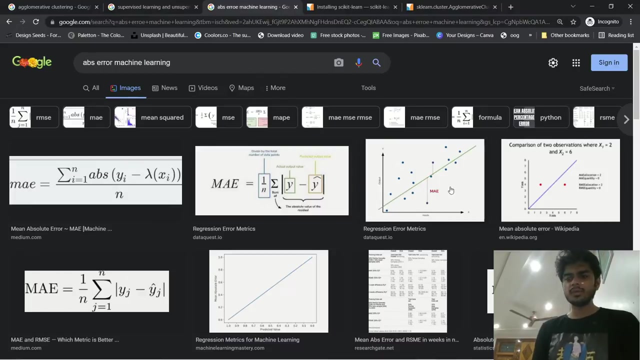 like explaining you, as we go through every like, we go through every uh terms which we find absolute error. so again like, what is absolute error? these all, these all are some fancy formulas for absolute error. so again it in: in very uh basic sense, it is about, like, how we can have our error minimized. 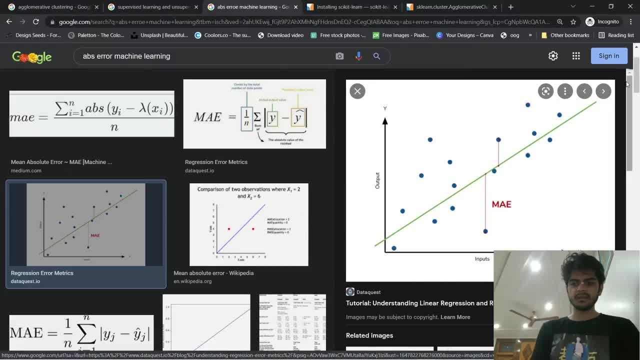 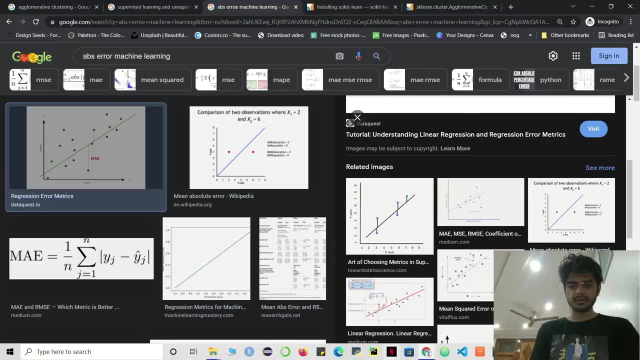 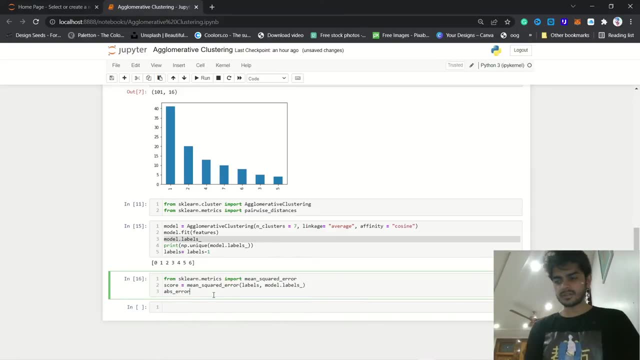 and again mean absolute error. this only, so it is a basically same thing: mean absolute error which we exp, which i explained like uh, like two, three minutes ago. so i will say: the mean absolute error is equals to np. dot, square root, sqrt or square root, and we will say: score. 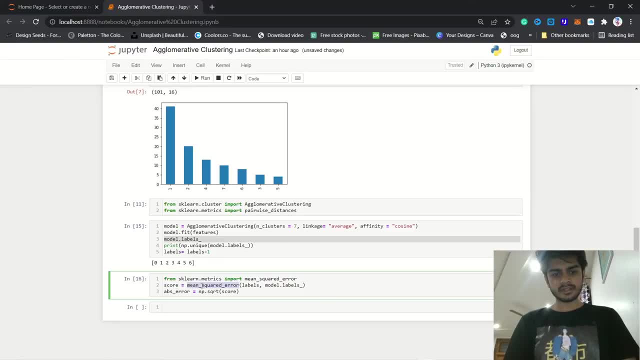 again, score is coming from this. we have took the mean squared error of these all terms. we're going got some values. then we will say that score like square root, that value which you got from these all thing, and then it will give us absolute error of that. and then we will. 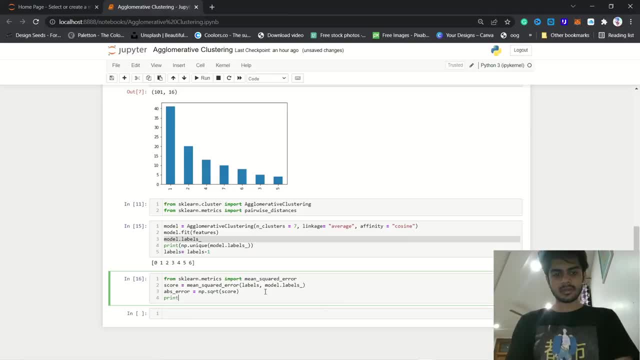 say, print that absolute error which we are working on. okay, and theoretically, what we should get is how good is our agglomerative plastic algorithm based on our all the data and the operation which we perform on our data, and how good and how better it is in.